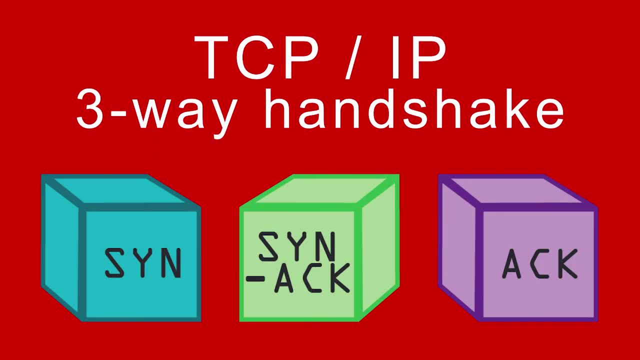 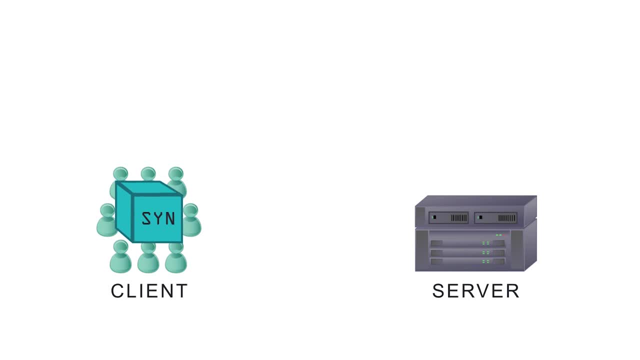 Another early trick involved exploiting the TCP IP three-way handshake. Here's how the handshake works: The client sends a SYN packet to the server indicating its intention to synchronize or start a conversation. The server returns a SYNACK packet acknowledging the SYN request. 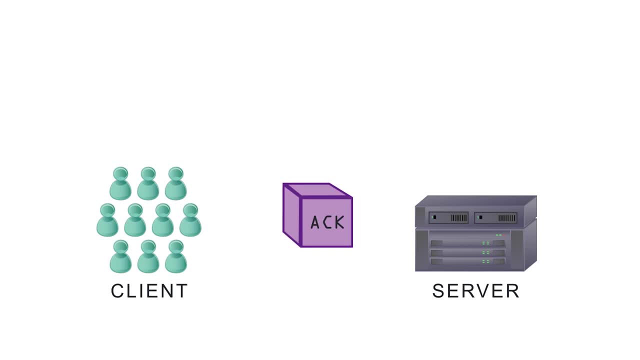 The client then sends an ACK packet acknowledging the SYNACK and waits for further communications. Hackers exploited this known process by not communicating after the final ACK, Which left the server hanging. The server is effectively left saying Hello, I'm waiting And waiting. 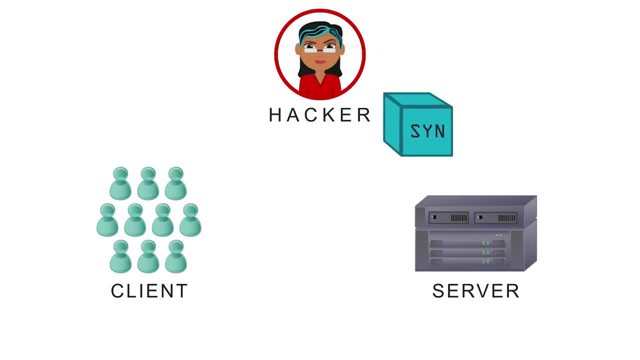 And waiting. The hacker starts multiple conversations and always leaves the server waiting after the final ACK packet. These fill the server's incoming queue and its limited number of open requests. The hacker has effectively backed up the server and denied service to all legitimate requests. 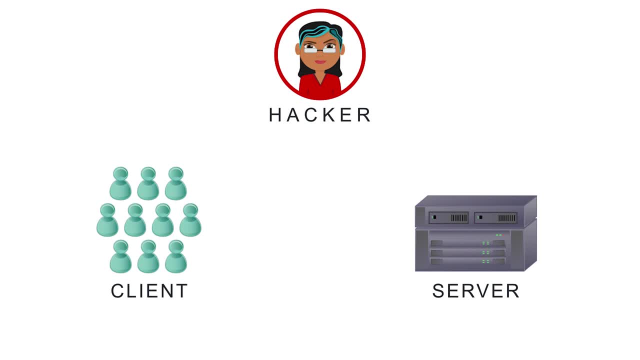 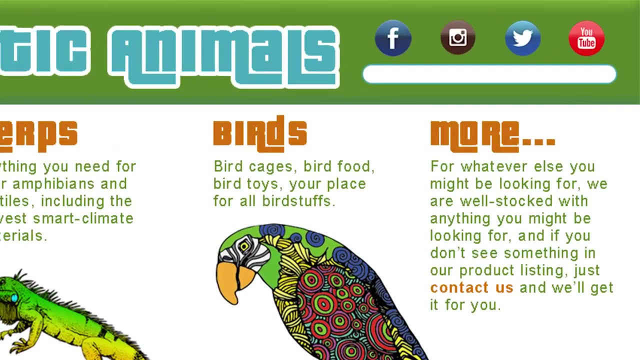 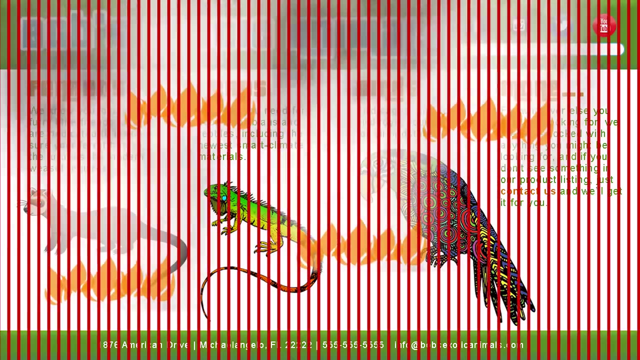 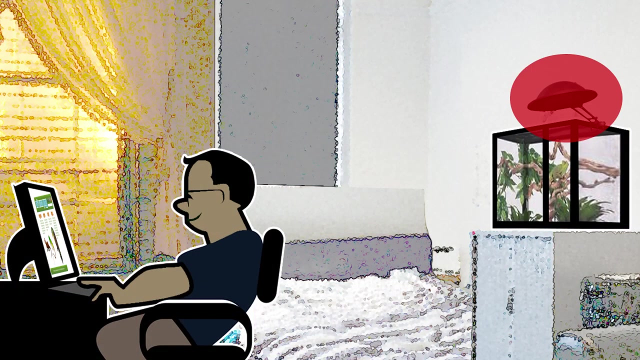 Aside from attacking TCP IP vulnerabilities, hackers are also adept at attacking poorly constructed websites. For instance, unprotected search mechanisms provide a popular point of access into a website. Let's look at a typical online store web application. Say you need to buy a heat lamp for your iguana. 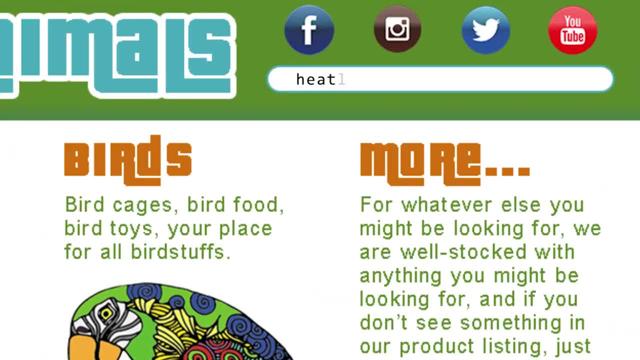 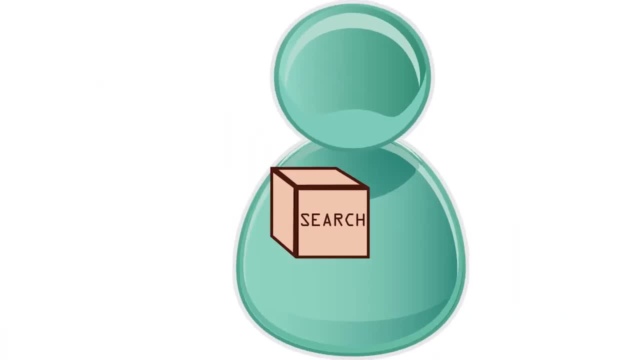 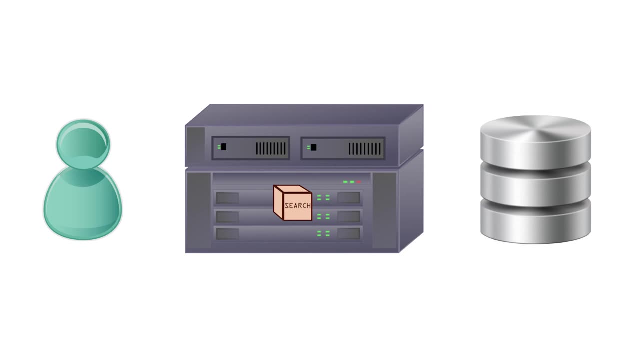 You enter the term HEATLAMP into the search box on Bob's Exotic Animals website, Your search request passes from your computer to the web server. But Bob's inventory isn't on the server. it's in his database. So the web server passes your search term to Bob's database in a query. 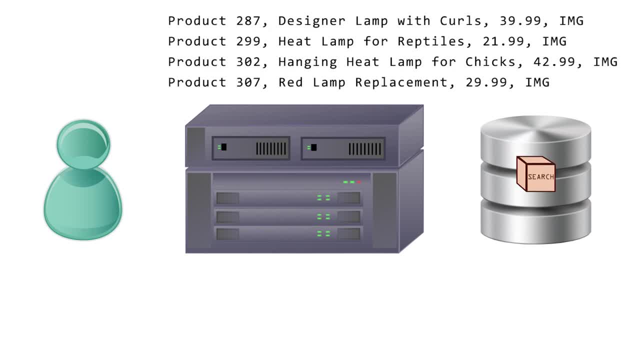 His database, compiles a list of all matching product records and passes it back to the web server, which organizes and formats those records before sending them back to you and displaying them on your computer screen. Ah, there's the heat lamp. Padfoot needs. 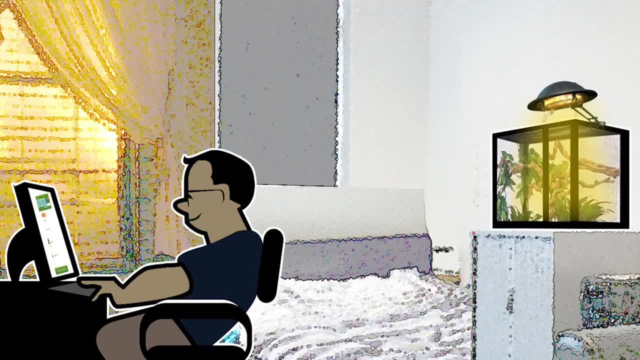 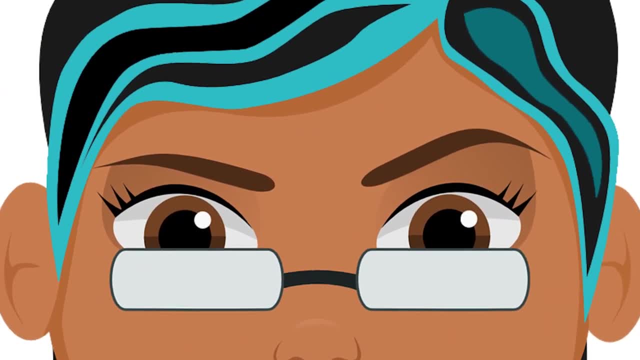 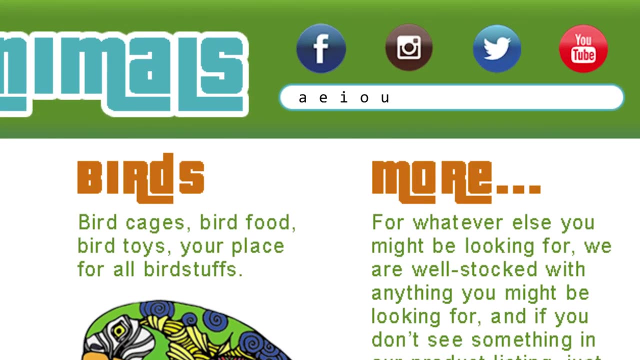 Legitimate searches like yours are no problem for Bob's website. But what if a hacker is attempting to crash the site? What if they're trying to trick the system into doing something it can't handle? Let's say the hacker enters A, E, I, O, U into the search box on Bob's website. 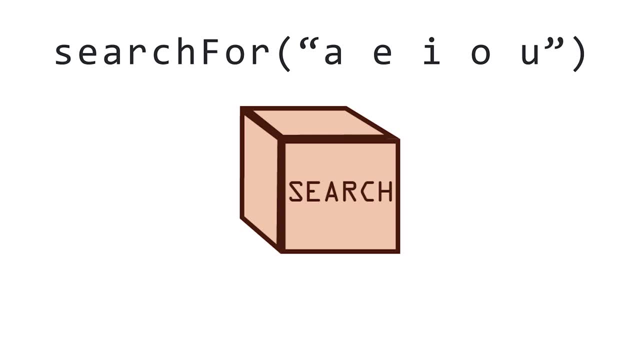 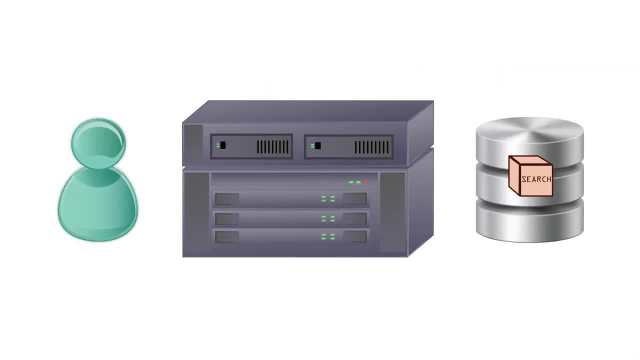 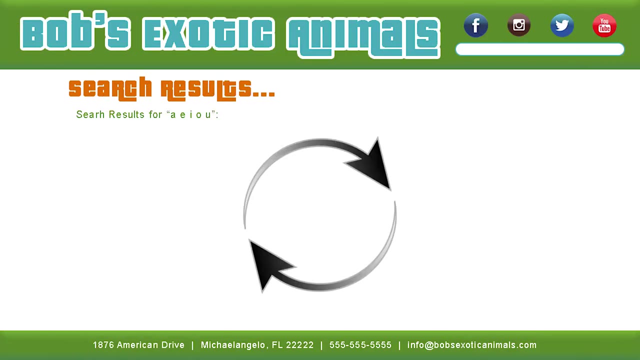 Instead of searching for a specific word or phrase, the hacker wants every product name that contains a vowel. The search request is passed off the same way to Bob's database. However, this time the matching product records take longer to compile because the hacker's request matches every product in Bob's database. 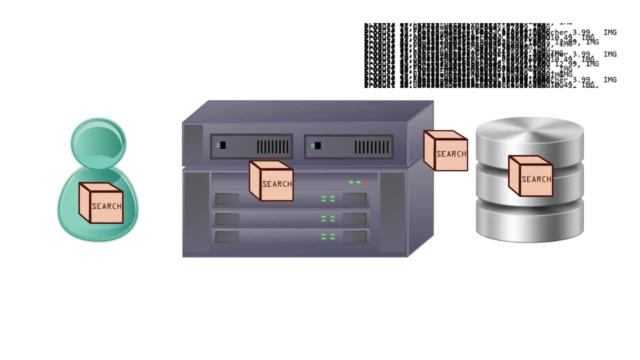 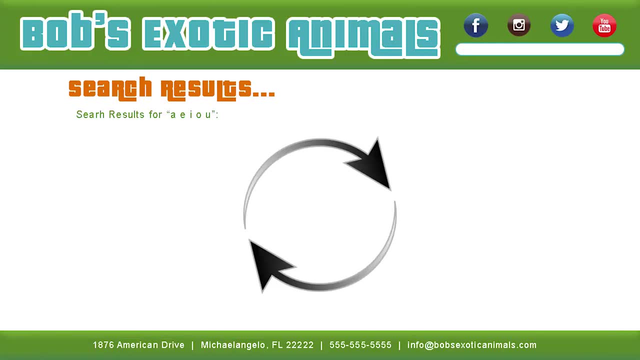 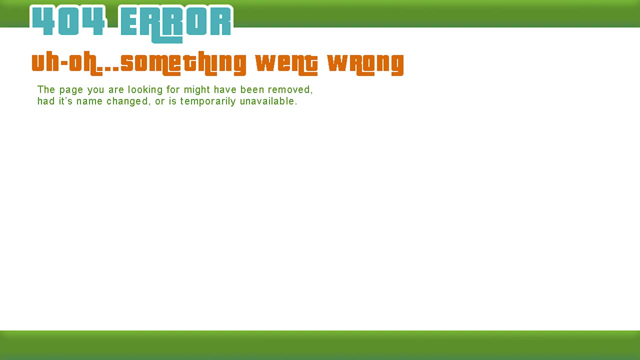 Now what happens if the hacker sends the same search request hundreds, if not thousands, of times? Because Bob didn't prevent this type of denial-of-service attack, it effectively locks up his database and shuts down his website. Now no one can order heat lamps. Nowadays, programmers design operating systems to address and avoid TCP IP errors. They also typically aggressively protect against malicious use of systems. Searching for the vowels A, E, I, O, U on any well-designed website won't fool the process and it won't take down a website. 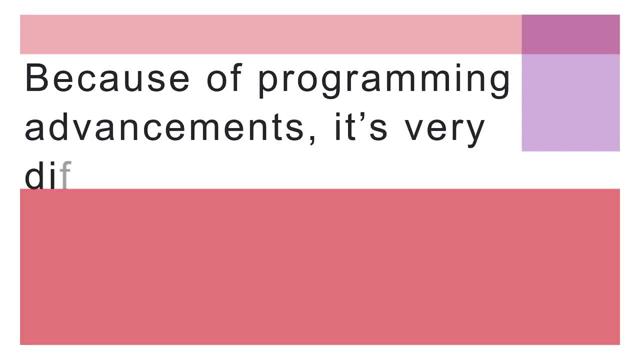 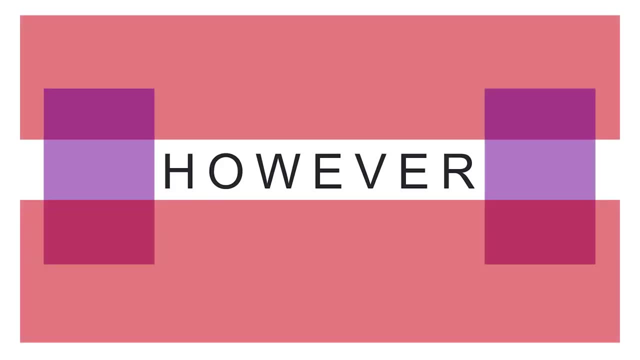 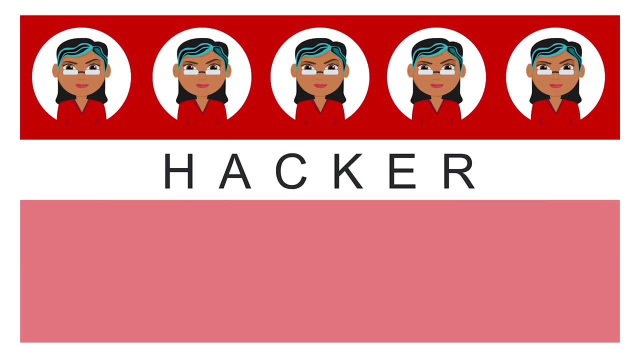 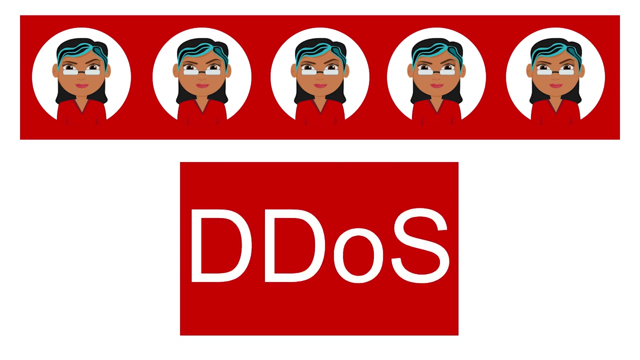 Because of programming advancements, it's very difficult for a single hacker to take down a server or network using these attack methods. However, as programmers address known vulnerabilities, hackers, ever innovative, continue to evolve and find new techniques to attack servers. DOS attacks have evolved into DDoS attacks or distributed denial-of-service attacks. 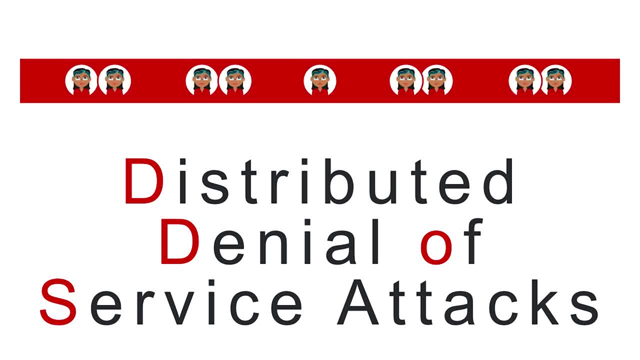 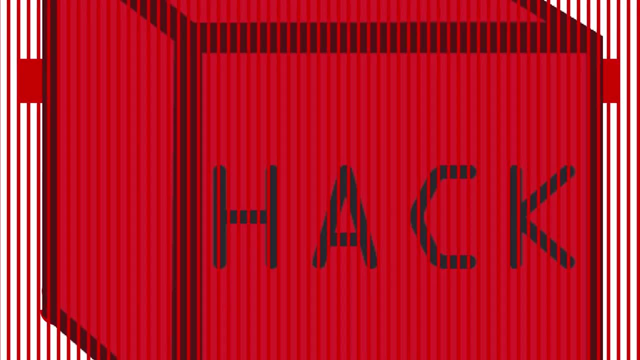 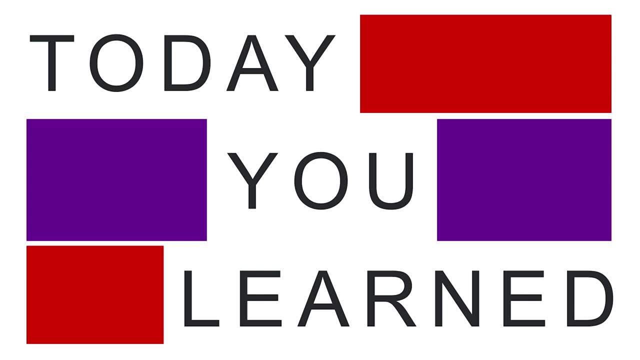 Distributed means the attacks are spread out over several, perhaps thousands of computers instead of launching from a single computer, But that is a topic for another day. Today you learned what a denial-of-service attack is and how hackers exploited early flaws in operating systems to deny service to authorized users. 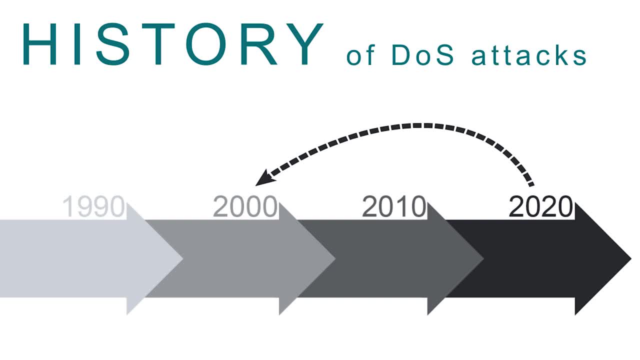 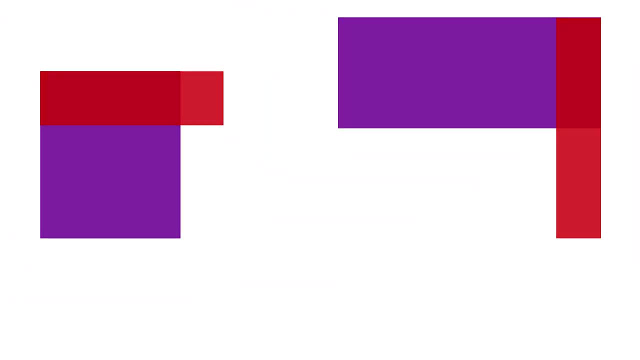 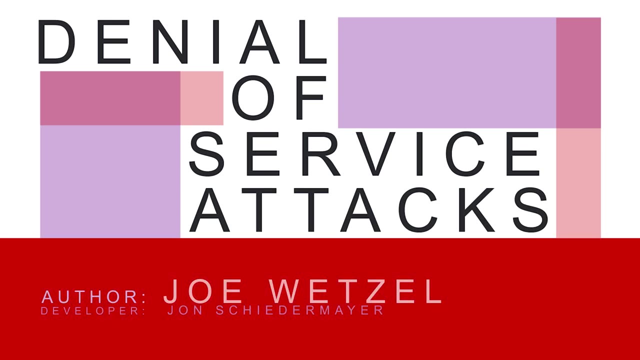 Understanding the history of these attacks provides you with the foundation to prevent future attacks. Congratulations, you've completed denial-of-service attacks. Thank you for watching.